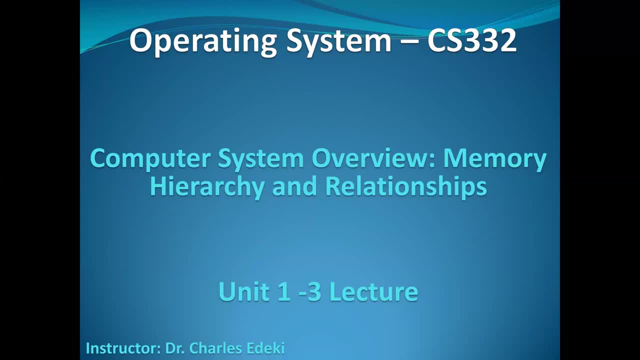 Again, welcome to operating system CS332 class. Again, this is computerized system overview and we're going to focus on memory hierarchy and relationships. As we know, in every computerized system there are different types of memory, from register cache all the way to the main memory. 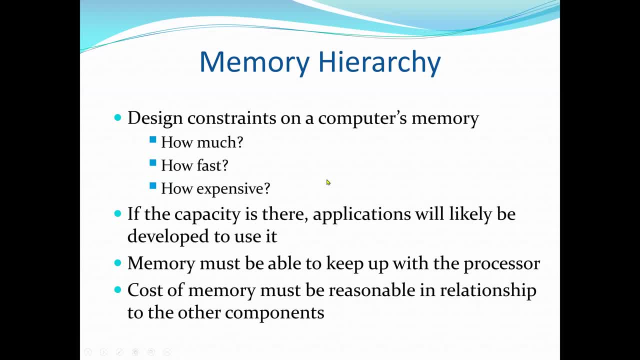 and we shall discuss the relationships between memory and also their hierarchy. And we know that the design constraints on a computerized memory can be summed up by three questions, And the three questions are: how much, How fast, How expensive And the faster the memory is. 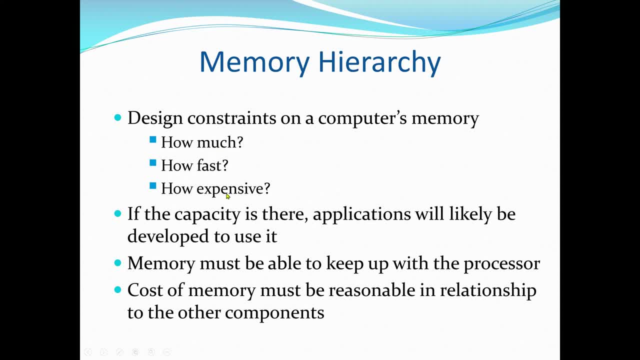 the less the amount and more expensive, The slower the memory. that means it will be less expensive and a lot. So we may answer these three questions. So now the question of how much is somewhat an open-ended question. We don't know how much specific value. 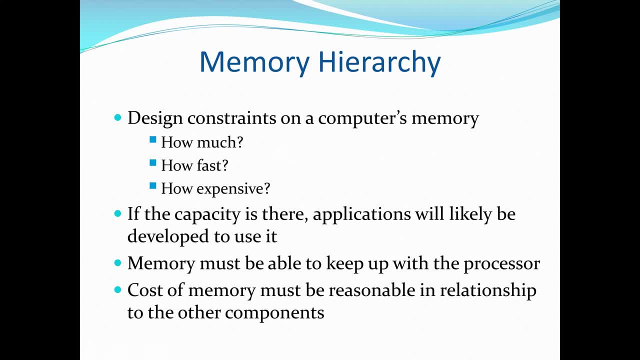 Now, if the capacity is there, then application would likely be developed to use it. Also, the question of how fast is, in a sense, is more easy to answer because to achieve it it's much easier to answer, because to achieve it it's much easier to answer. 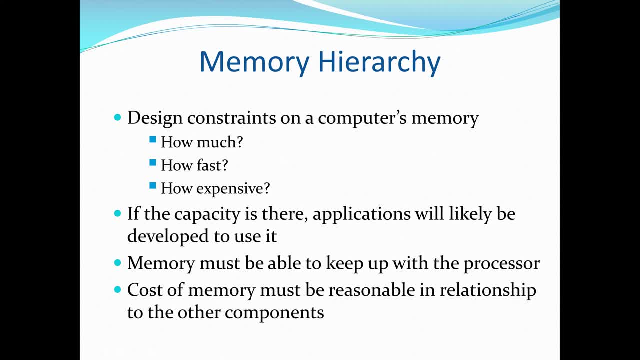 to achieve the greatest performance, the memory must be able to keep up with the processor, That is, as the processor is executing instructions, we will want also the memory to be providing enough information at a constant rate with the processor. Otherwise it will reach a stage whereby the processor 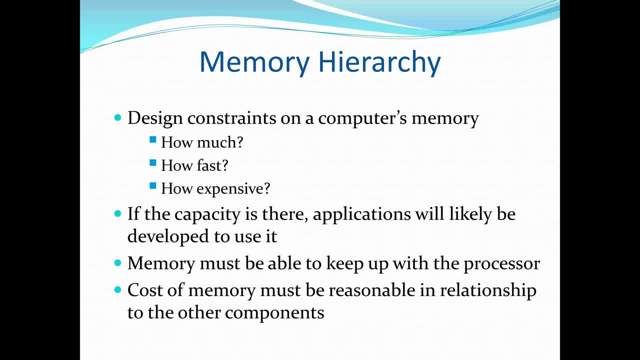 will pause or stay idle because there's no data information if the memory is slower. So here we say: if the capacity is there, application will likely be developed to use it Now. memory must be able to keep up with the processor. 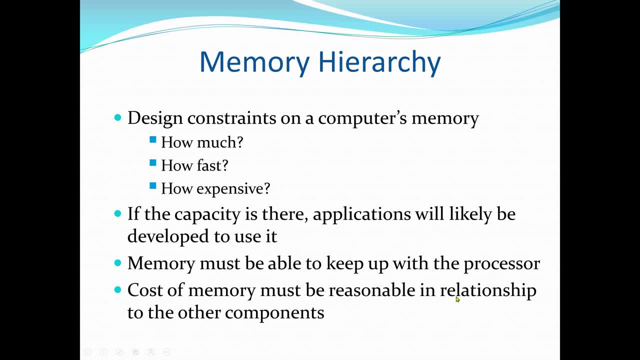 And now the cost of memory must be reasonable in a relationship to the other components. And that was again our final question. We need to consider the cost. So for a practical system, the cost of memory again must be reasonable in relationship to other components. 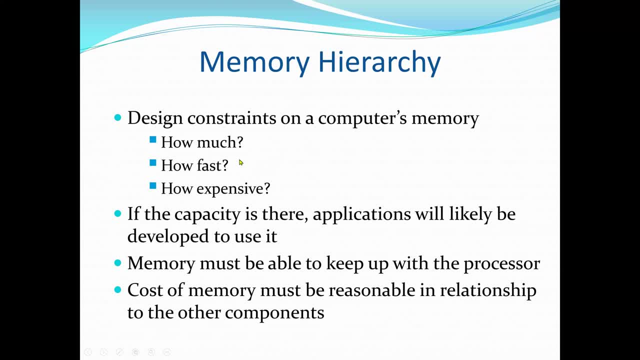 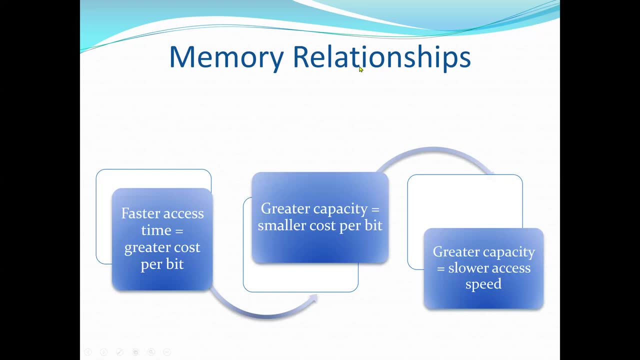 So this is the concept of memory hierarchy. We're going to consider these three characteristics, So I'll say the three questions of the memory: How much, how fast and how expensive. So again, memory relationships. we can see here the faster access time. 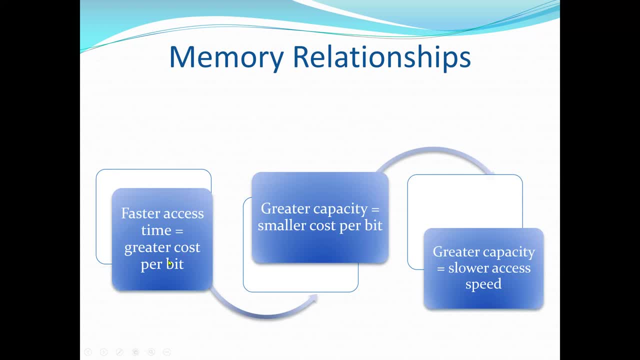 equal to what the greater cost per bit. So if the memory is faster to access by the CPU, then the cost will be higher, as we said earlier, And also the greater capacity goes with the smaller cost per bit. So the higher the larger the memory. 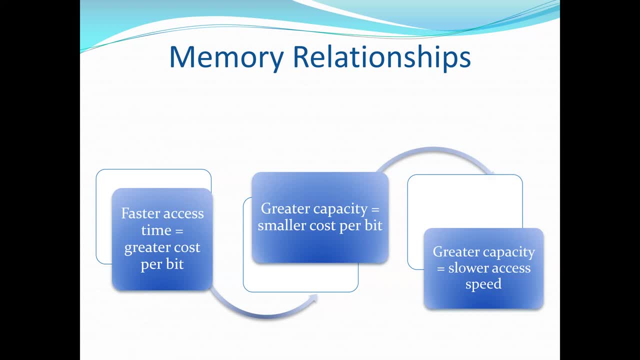 the cost may go down, but the speed may slow down. So here also we say the greater capacity equal to slower access speed. So, as might be expected, there's always a trade-off among these three key characteristics of a memory: The capacity, access time and the cost. 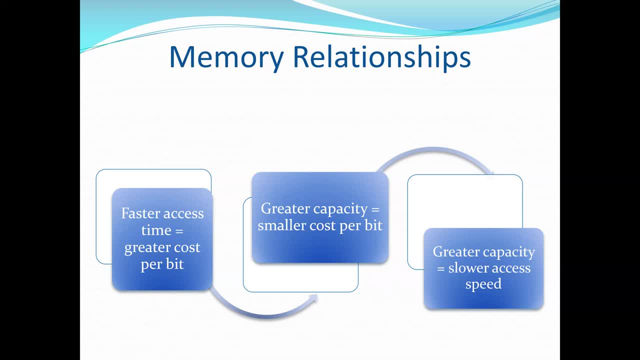 And those are the three questions we were asking before. So a variety of technologies are used to implement memory systems And across this spectrum of technologies, the following are the most important. The following relationships hold: Faster access time. greater cost per bit. 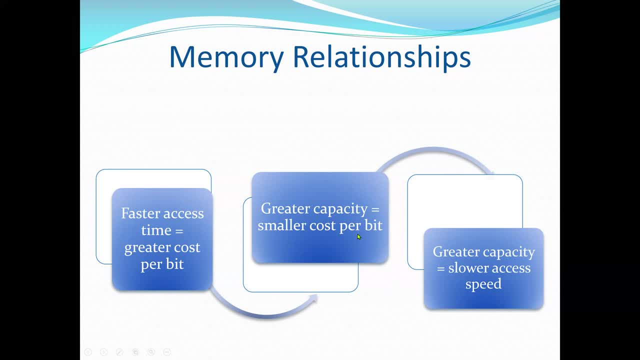 Greater capacity, smaller cost per bit And also greater capacity, slower access speed. So the dilemma here is that we are facing here is very simple or very clear to the designer. The designer would like to use memory technology. the designer would like to use memory technology. 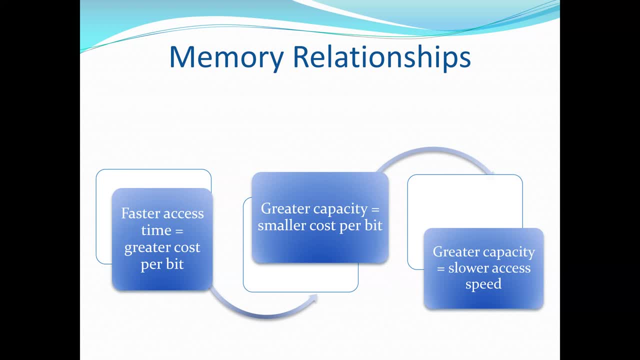 and the low capacity memory, And in fact, these are the main technologies that provide for, again, large capacity memory, both because the capacity is needed And also because the cost per bit is slow. However, to meet the performance requirements also, the designer needs to use expensive one. 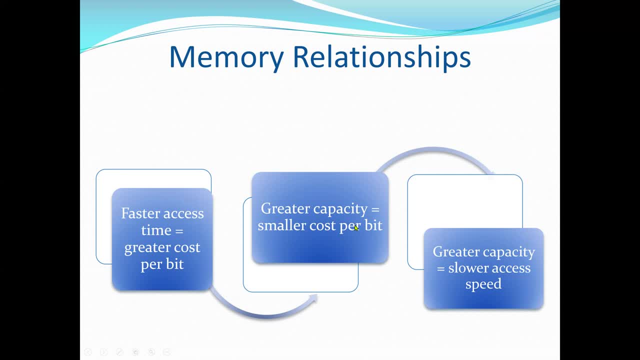 relatively lower capacity memory with faster access speed. So I would say the difference between the main memory, which is more larger but slower to access by the processors or CPU, are greater and lower capacity memory you comparing to cache, which is closer to the to the cpu, so faster to access. but 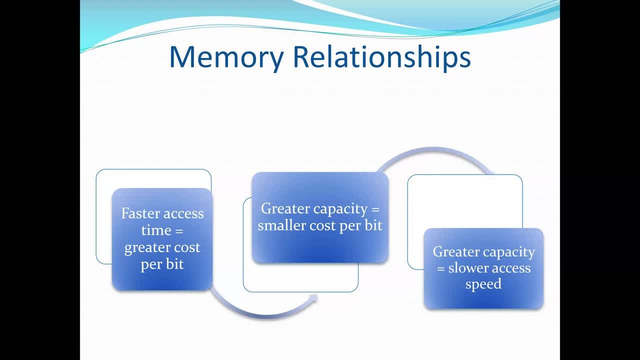 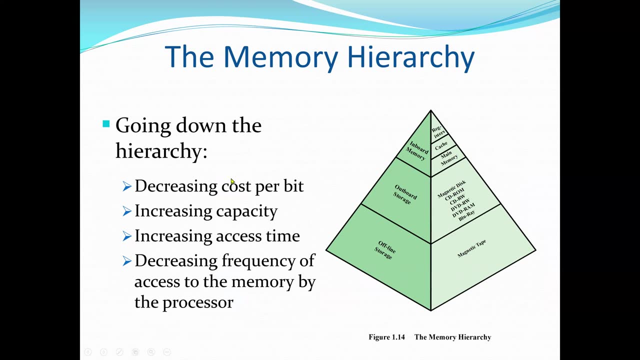 very expensive, so it must be less memory. the capacity must be less. so this is our memory higher ranking going down the higher ranking: first of all decreasing cost per bit, then increasing capacity and then increasing access time, decreasing frequency of the assets to the memory by processor. so here we have the inboard memory, then outboard storage. 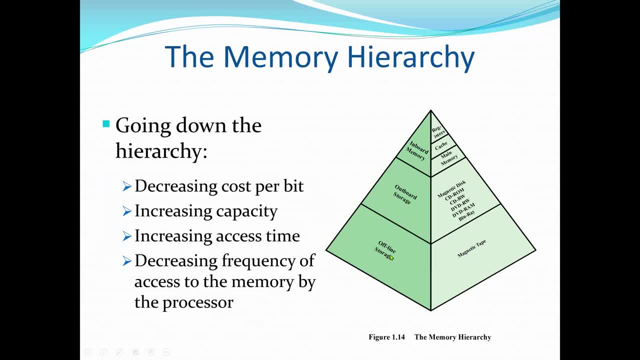 then offline storage, which will be more slower and also so from the higher it's more faster and less capacity and most expensive. so one will be the registers which are normally some of designers have. the registers inside the cpu. caches will be next to the cpu, their main memory. this is where this is the only place. this is called the inboard memories. 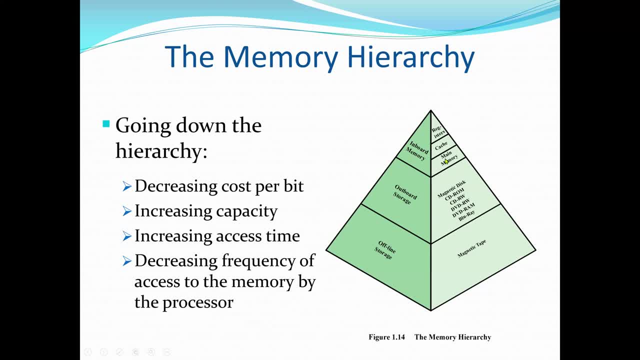 the computer. this of the cpu can only access these three types of memory. then we have the outboard storage, like again, cd-rom, the hard drive etc. but the cpu cannot access any of this. so in order to execute a program or any task, the program and the data must be loaded to the main. 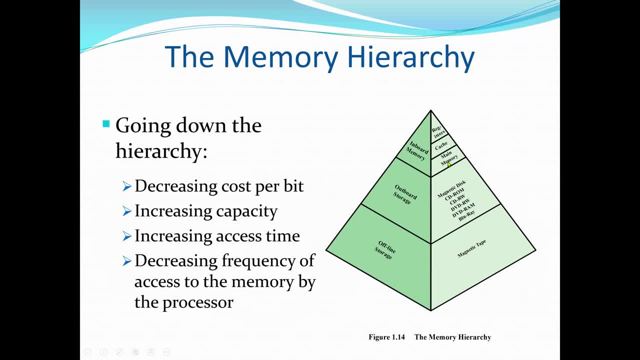 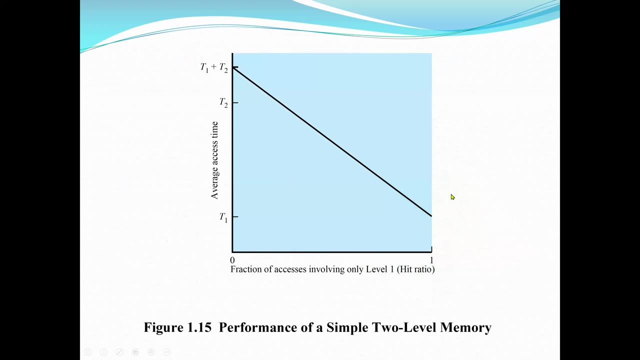 member cpu can access the main memory, but it's very slow. we may discuss this more detail when we start main memory chapter. so, as we expected, again, there's always a trade-off among all the tricky characteristics: the capacity, the asset stand and also the cost. now, the way out of this dilemma is to not rely on only one single memory component. 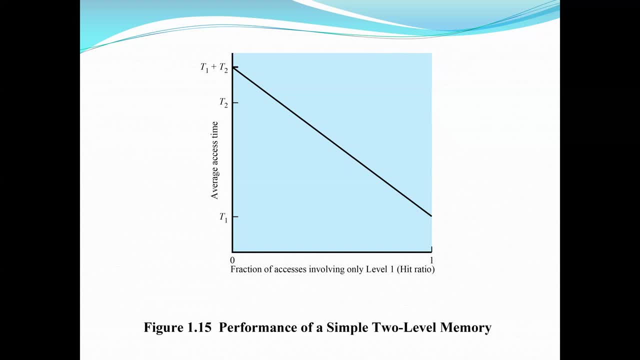 or technology. so we see most of our computer system today. we have all the three type of memory in our computer. we may have a register inside the cpu, the chip. then we may have a cache very close to the cpu, then the main memory, a little more far, far away from the cpu. 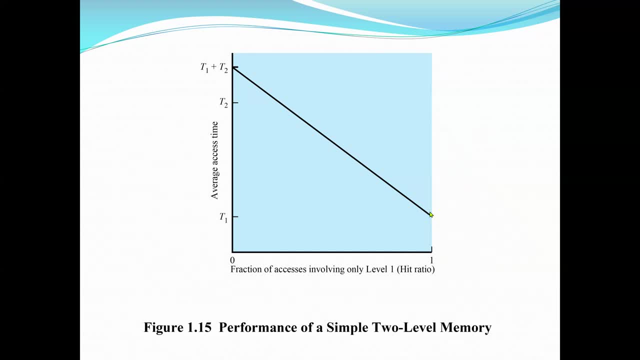 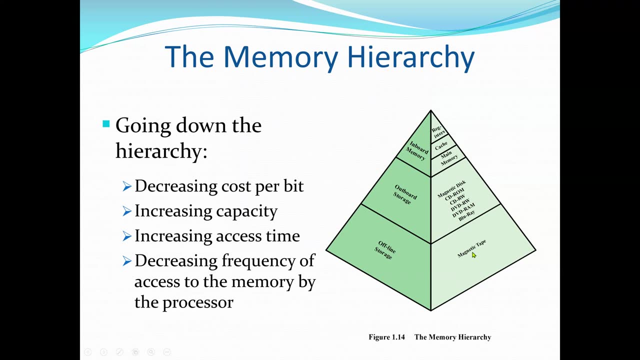 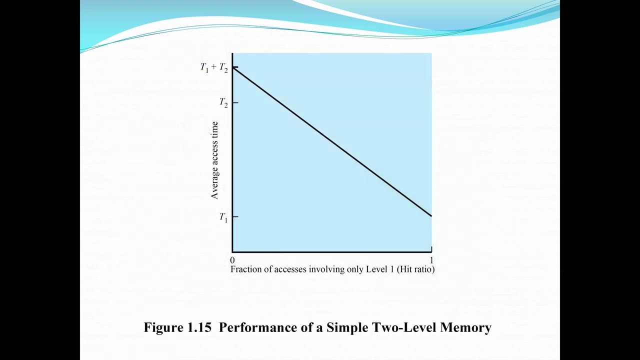 so a typical rank is, as we saw the illustration again from memory, or the, so the down is more slower, which is the magnetic tape. this way we can look for the so-called. so let me show you a simple two-level memory. so this again, we can see the diagram performance of a simple two-level memory. 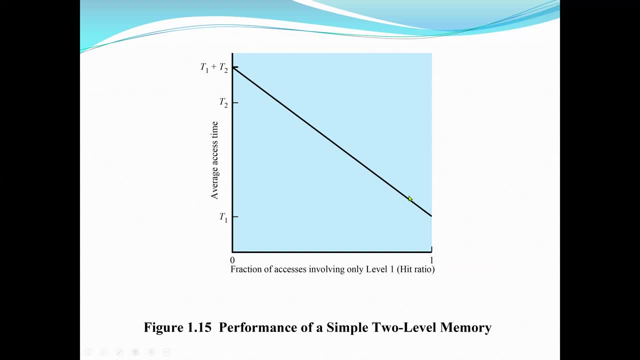 and we have the fraction of assets involving only level one heat ratio and also the average. Now suppose that a processor has access to two levels of memory, which again is level one containing 1,000 bits and has an access time of 0.1 microsecond. 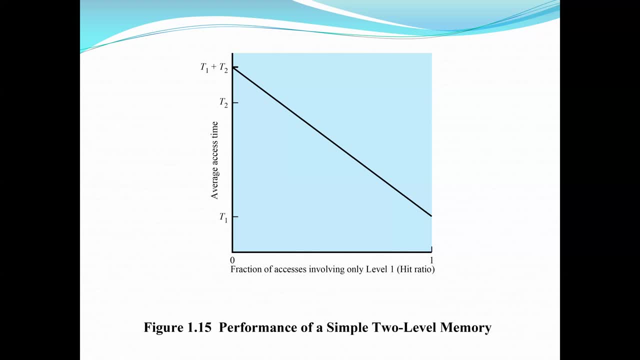 Level two contains 100,000 bits and it has access of one microsecond. Now, assuming that if the byte to be decreased is in level one, then we know the processor accessing it directly. Now, if it is in level two, then the byte is first transferred to level one and then accessed by the processor. 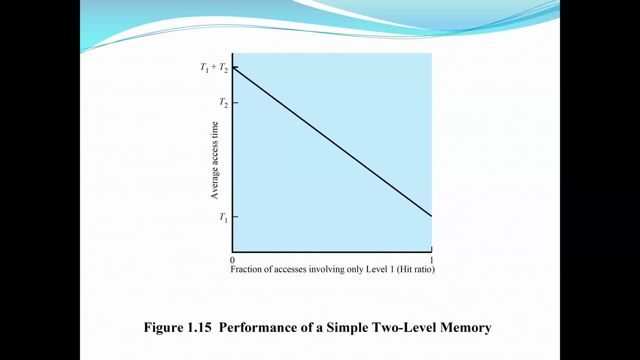 So for simplicity, we can ignore the time required for the processor to determine whether the byte is in level one or two. That's the concept here. again, Main memory or the data programs are loaded there when we open our program or data. Now for the CPU. we want to transfer: 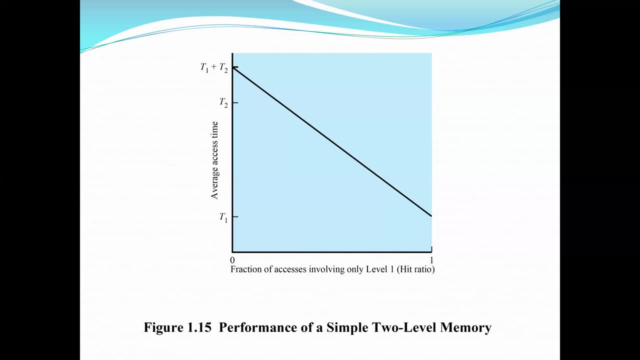 The data from the main memory add up to the cache, which is next to the CPU, then from there to the register, which is another memory inside the CPU. So register will be holding the data or the program that is being executed during execution time. 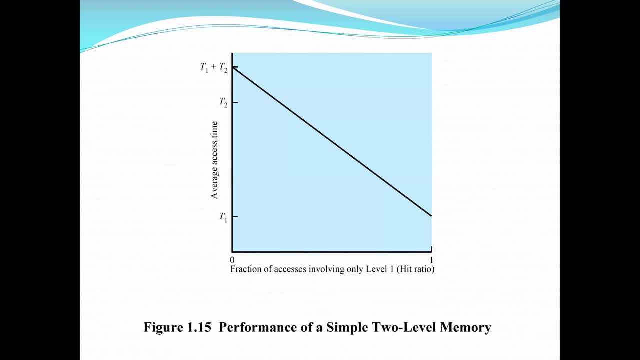 Now suppose that the processor has access to two levels of memory. So we say level one, We have two. So level two zero and one contain 1,000 bytes and has access time of 0.1 microsecond. 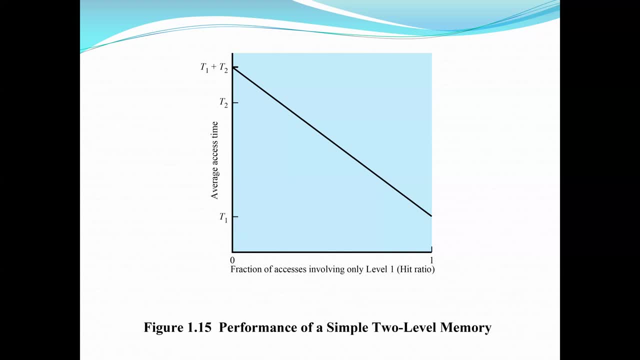 And also level two, contains 100,000 bytes and has access time of one microsecond. Now, assuming that if a byte to be accessed is in level one, then the processor also can access it directly, But if it's in level two, then the byte is first transferred to level one, then accessed by the processor. 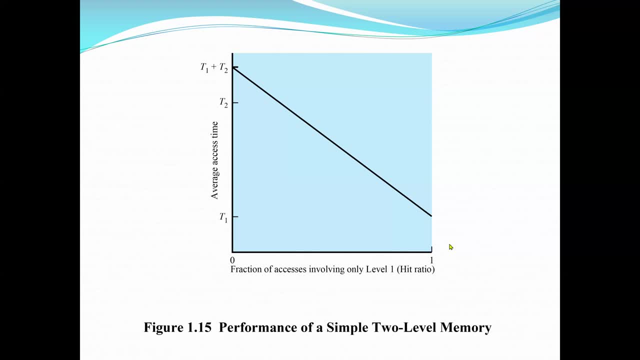 So here, And this diagram shows general shape of a curve that model the situation, We can see that the figure shows average access time to a level two memory as a function of heat ratio, which is the heat ratio where heat again is defined as the fraction of all memory assets that are found in the faster memory. 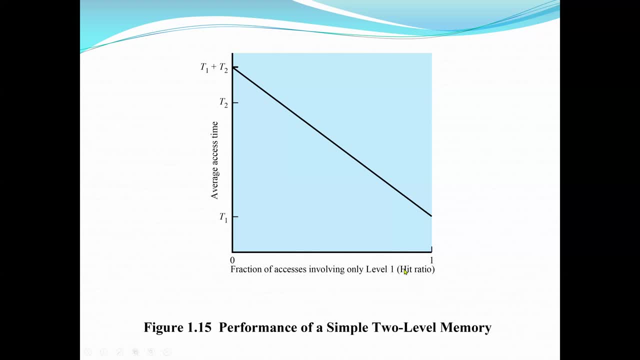 Example can be the cache. Now, T1 is the access time to level one, So we can see very shorter time, And T2, which is more longer, is access to level two. As can be seen for a higher percentage of level one access, the average total access time is much closer to that of level one than of level two. 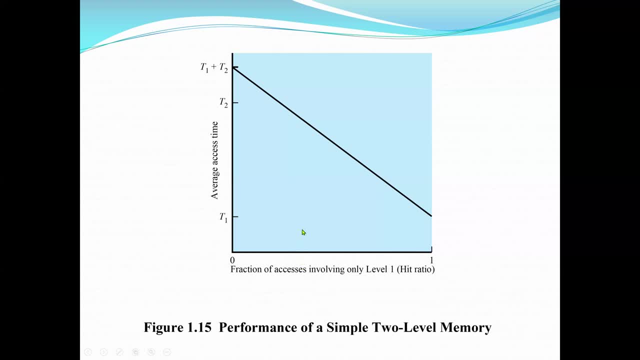 So in our example here, suppose 95% of the memory is in level two. So we can see that the average total access time is much closer to that of level one than of level two. So we can see that the average total access time is much closer to that of level two. 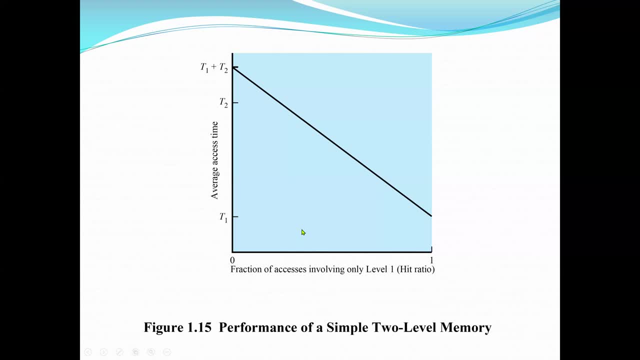 So we can see that the average total access time is much closer to that of level one than of level two Of rather a memory assets found in the cache. Let's say h equal to 0.95, or 95%, Then the average time to access the byte can be expressed as, again, the time was 0.1 seconds. 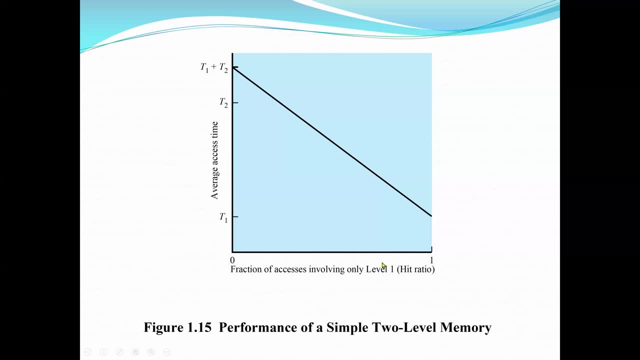 So it will be 0.95 times 0.1 second plus 0.05 times 0.1 seconds plus one second, which in all it will give us roughly somewhere around 15 seconds: 0.1 seconds plus 1 second. 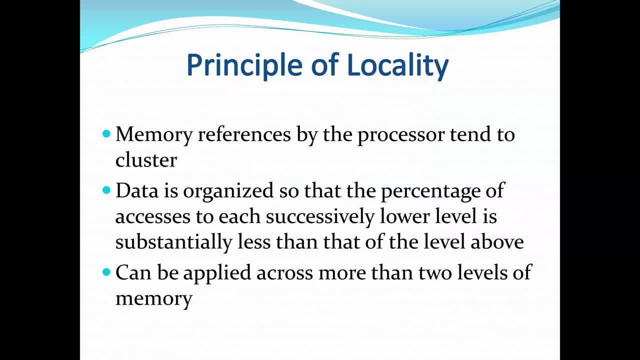 So it will give us roughly some amount of nostra hora. So it will give us roughly some amount of nostra hora somewhere around 0.15.. So the result is close to the access time of the fast start memory. So using the average, So the strategy of using two memory levels work in principles, but only. 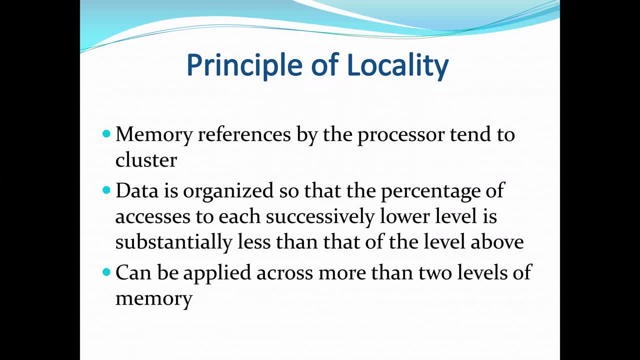 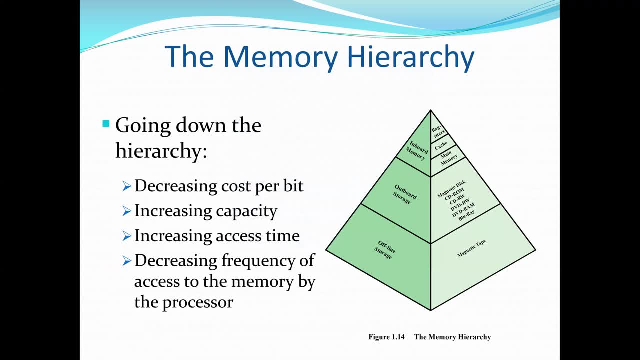 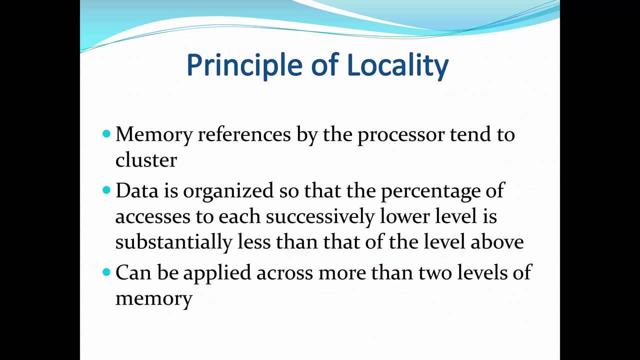 if the condition A through D in the preceding list apply- And that was the previous condition here- The cost, capacity, time and also the frequency of access. Now, next, we go to the concept of principle of locality, So the basis for the validation. 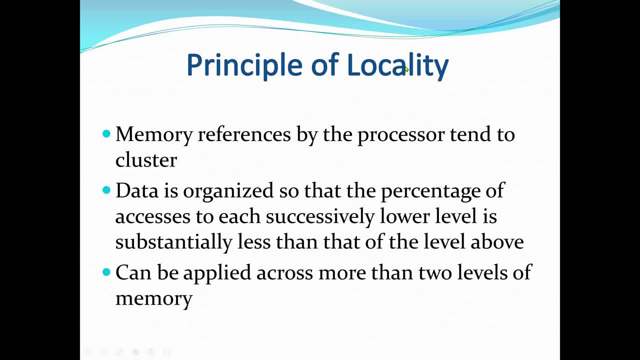 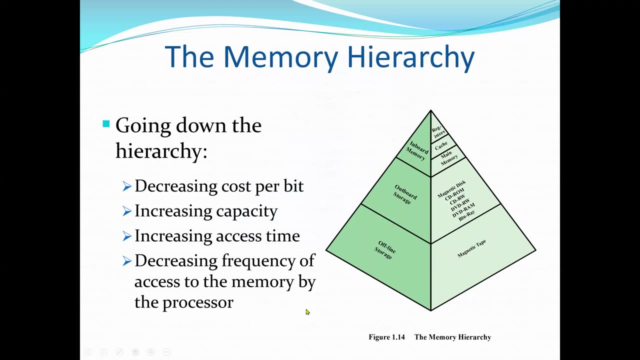 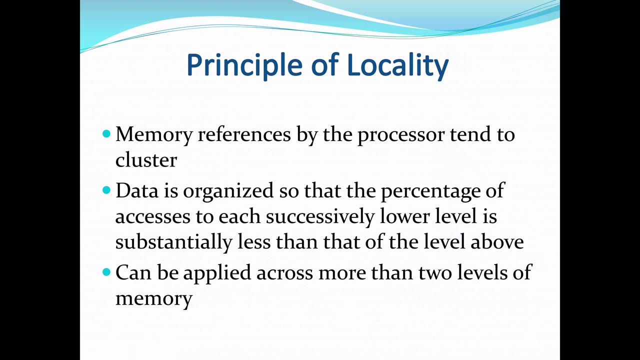 or validity of a condition. D is the principle known as locality of reference or the principles of locality. Here we talk about the frequency of access to the memory by the processor. So during the course of execution of a program, the memory references by the processor tend to. 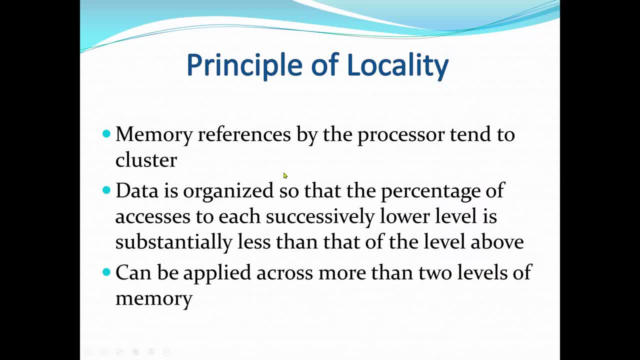 cluster, Then pull for the instructions and data Again. they tend to cluster, as the memory references by the processor tend to cluster for both instructions and data. Now, programs typically contain a number of interactive loops and subroutines. so once a loop or subroutine is entered they are repeated references to small sets of instructions. 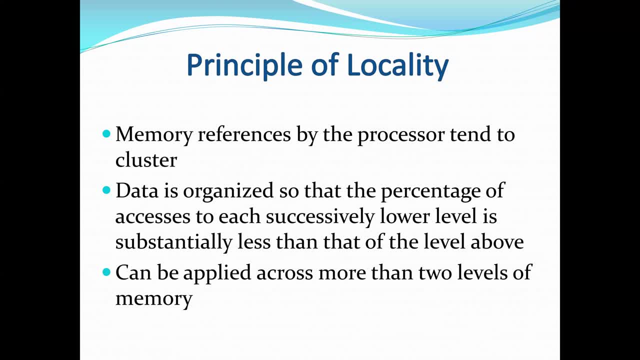 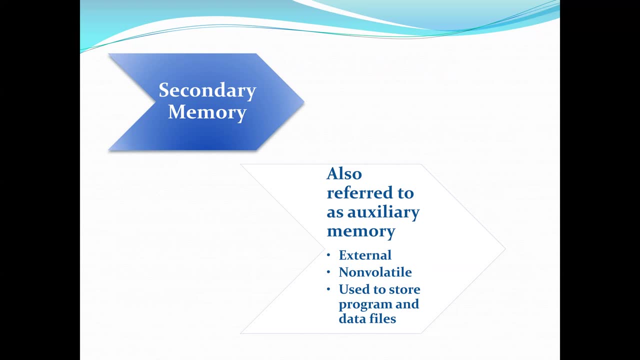 So, similarly, operations on tables and arrays involve access to the cluster set data, just like the same script structure, Now over a long period of time. now we can notice that the cross-stats in use will be changing, but over a short period of time. 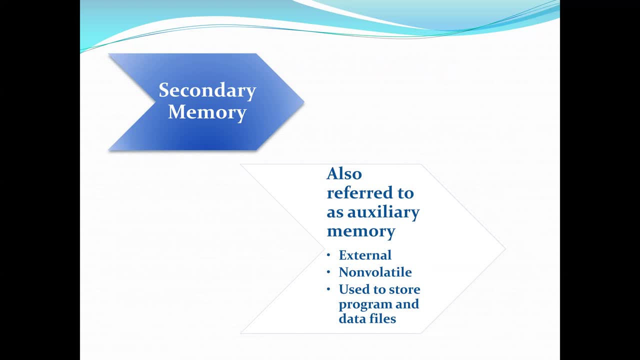 So the processor again is primarily working with phase cross-stats of memory references. Now we have three forms of memory, the major three forms. I'm just going to describe One thing we know about memory. we have the one that is volatile. Volatile means when the data is, power is off, the data are lost. 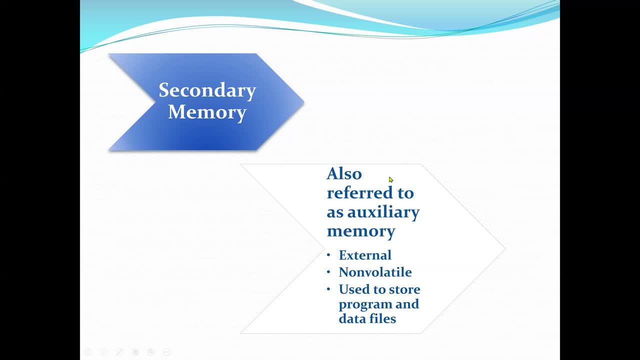 So we have secondary memory, which also refer to as auxiliary memory. This will be external, can be external like a flash drive, hard drive, external hard drive. It's non-volatile because if computer is not working it's not going to be able to. 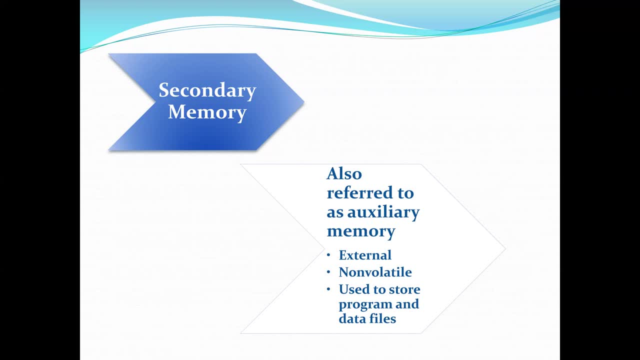 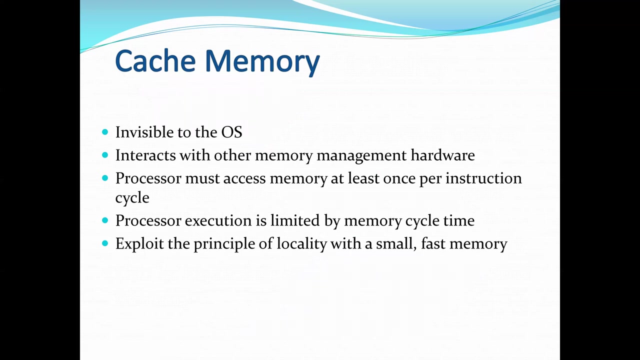 switch on and I save my data. if I turn the computer off, the data will still be there and normally used for stored programs and data files. Now we also have the cache memory. Now the use of the three levels is where the fact that semiconductor memory comes in variety. 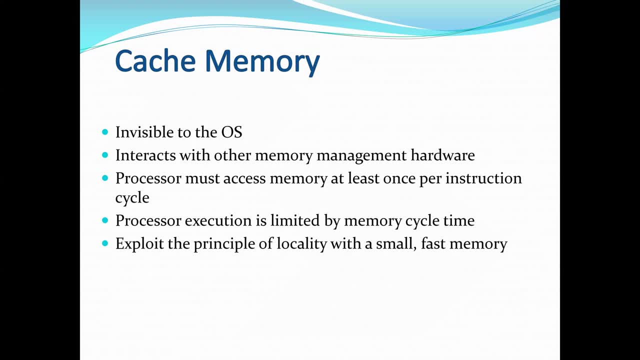 of types and we will discuss these more details when we cover memory lectures and also virtual memory, That's memory management. So cache memory. although we say that cache memory is invisible to the OS, still it interacts with other memory management hardware. So, invisible to the OS but interact with other memory management hardware. 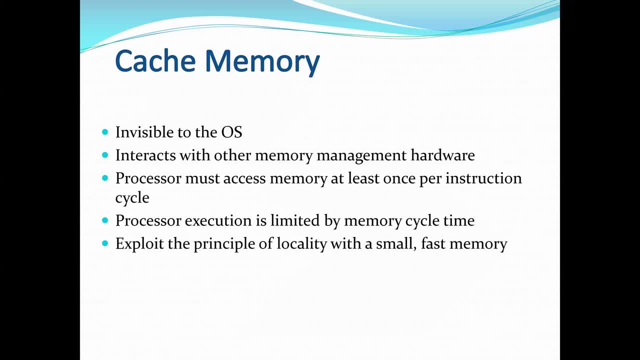 Furthermore, many of the principles used in virtual memory schemes, which we are going to discuss in chapter eight of our course Testbook, are also applied to cache memory. So on all instruction circles, the processor normally access memory at least once to fetch the instruction and often one or more additional times to fetch operands and all stored results. 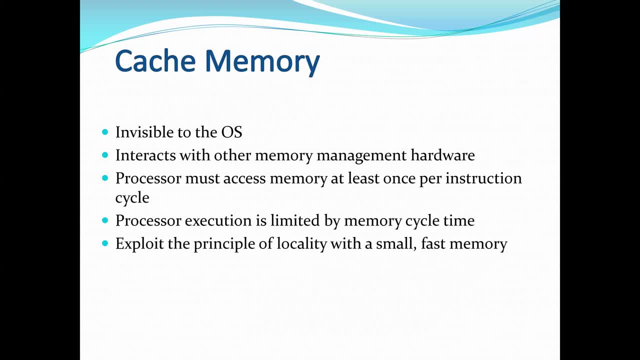 So the rate at which the processor can execute instruction is clearly limited by the memory cycle time. That's the time it takes to read, Read one word from or write one word to a memory. So here we're going to explore the principles of locality with a small, fast memory. 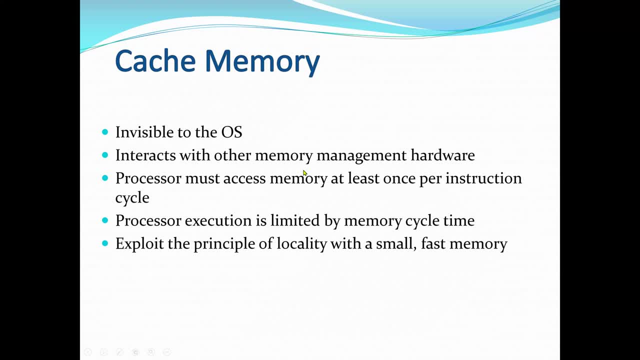 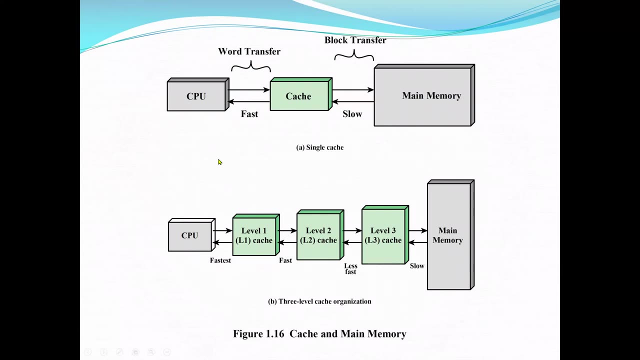 Because again, processor execution normally is limited by the memory cycle time. So we can see again from the diagram we have, And here we have the memory cycle time, And here we have the memory cycle time, And here we have the CPU. As we said earlier, we can see where the main memory is. 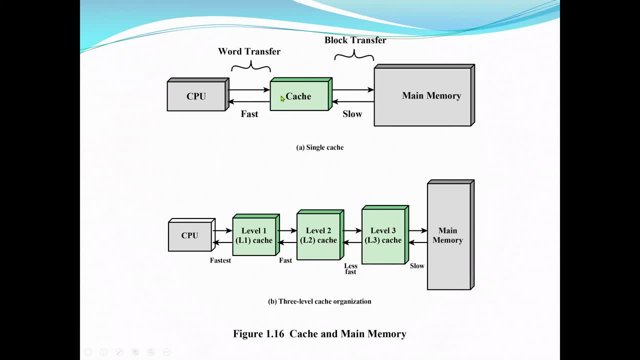 So the cache is more faster for the CPU to access. So we say fast, but the CPU to access data or instruction for main memory is very slow. Now we can see our second diagram. We have different, as we said, different levels of caches or even a register which can be. 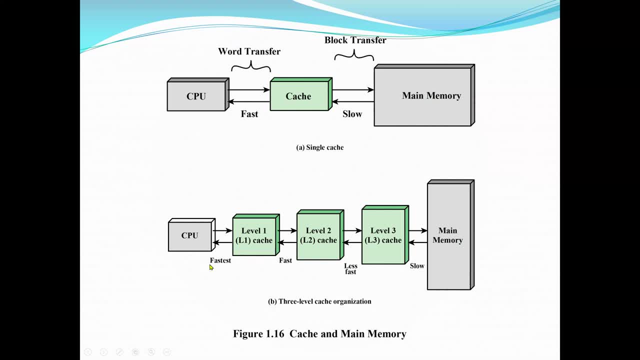 inside the CPU, So it will be more faster. So level one will be fastest, level two fast. level three: less fast than main memory access, Very slow. So cache memory is intended to provide memory access time approaching that of the fastest memories available. 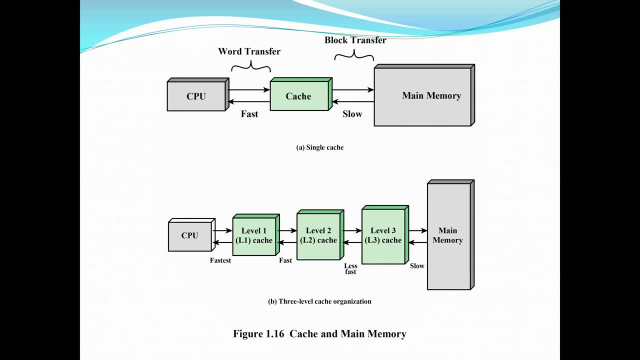 Also, at the same time, support a large memory size. That has the price. That's the price. That's the price of less expensive types of semiconductor materials. So we know level one cache is more expensive. So we can see the size of the memory by using the box size. 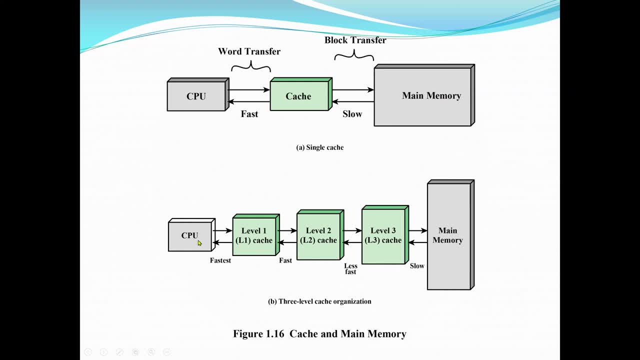 The faster the memory that is closer to the CPU, the less the capacity, because it's too expensive to beat. So So So the concept: again it shows in these two diagrams here. So there's a relative large and slow memory together with small, faster cache memory. 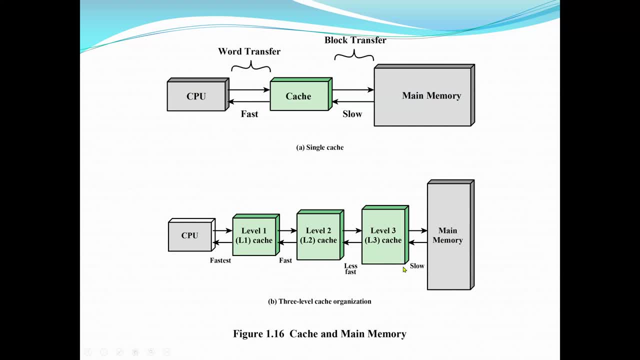 Almost every computer designs look something like this: as we said, maybe have a register in the CPU, which is also a memory which again very close to the CPU. the closer the memory to the CPU, the faster the CPU can access it. 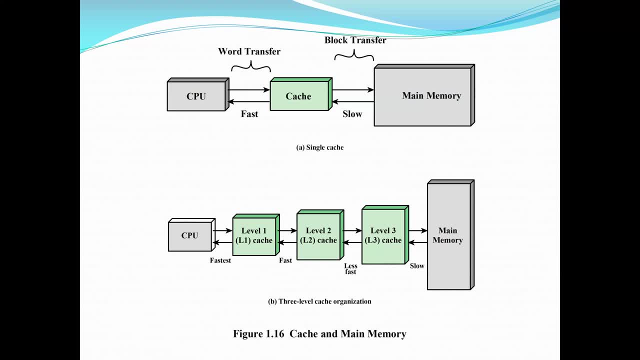 So when the processor attempt to read a byte or a word of memory, a check is made to determine if the byte or word is in the cache. If so, the byte or the word is delivered to the processor. If not, a block of main memory consisting of the same face normal byte is read into. 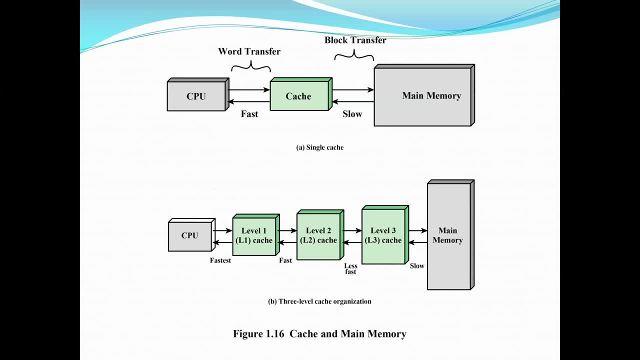 the cache and then the byte or word is delivered to the processor. This is what takes. It will take more time. So, because of this phenomena of locality of reference, when a block of data is fetched into a cache to satisfy single memory reference, then it's likely that many of the near future 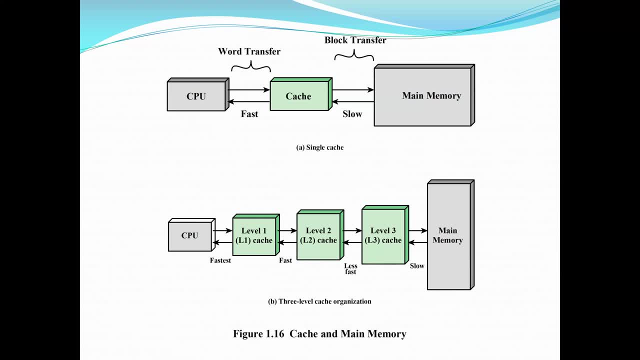 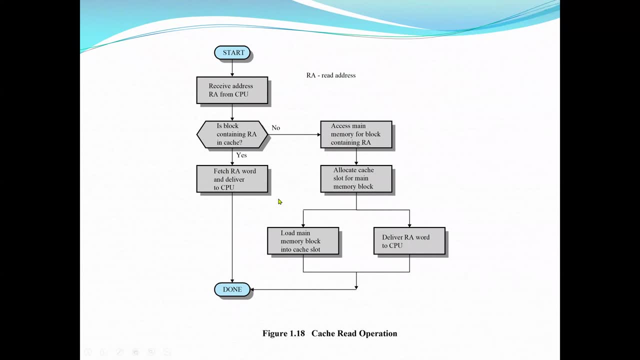 memory references will be to the other bytes in the block. So This is the concept here. This diagram will illustrate the read operation. You can see the process again. generates the address RA. read address RA. receive address RA. That's the start from the CPU. 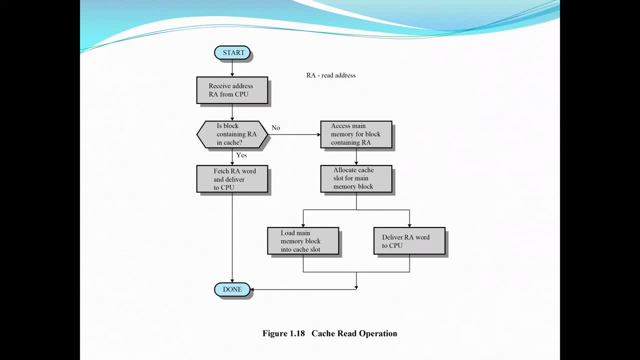 Then if the word is contained in the cache, it will be delivered to the CPU. If not, then we go Otherwise: the block containing the word is loaded to the cache And again they'll deliver to the processor. So we can see the flow diagram here. 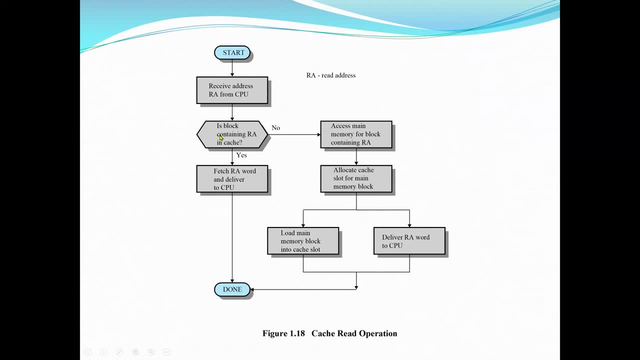 Start. receive address RA from. the CPU Is block containing the RA. That's the read address in the cache. Yes, If yes, then we fetch the RA word to deliver to the CPU. Then we are done More quicker. But if no, then we have to access the main memory. 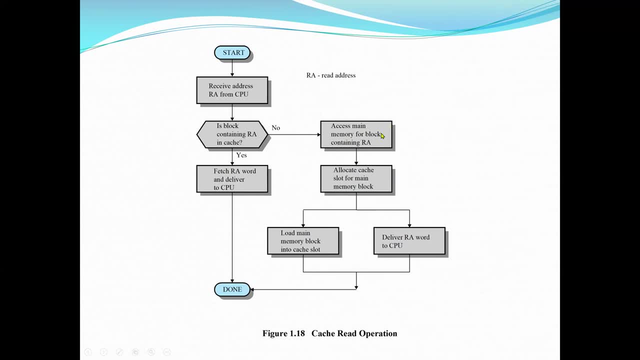 For the block containing the read address. That's the read address in the cache. Yes, If yes, then we fetch the RA word to deliver to the CPU. Then we are done read address array. then we allocate a cache slot for the main memory block. 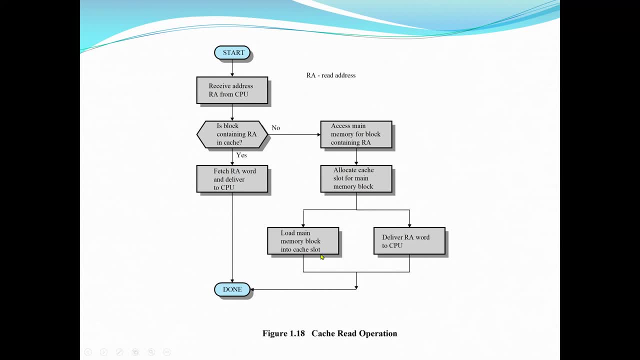 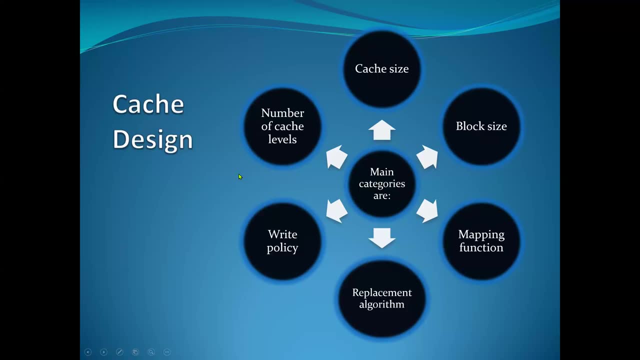 so then we load the main memory block into the cache slot, then we deliver it to the cpu. so we have different types of uh cache, as we saw- level one, level two- but they are the same design. okay, the difference is the speed, access time. so if we are designing a cache, these are the elements, or the key elements, that we have to. 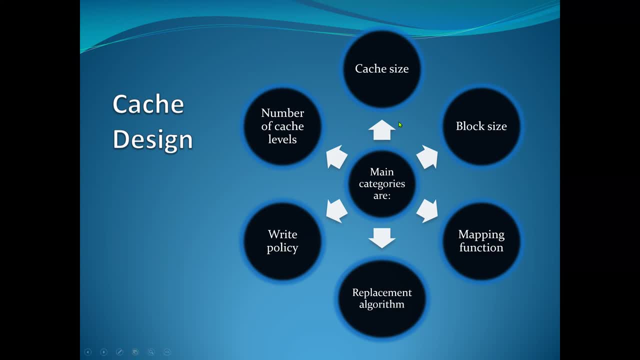 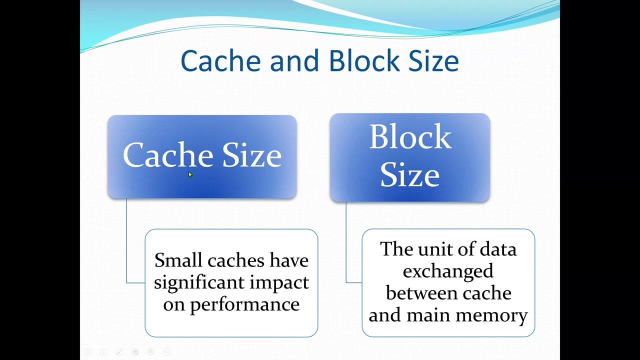 consider. we should consider the cache size, the block size, the mapping function, and then replacement or guaranteeing, and also the writing polities a policy, the right policy, replacement or guarantee, mapping function. so we'll go through each of these. so the cache and the block size. so here we say the cache size. 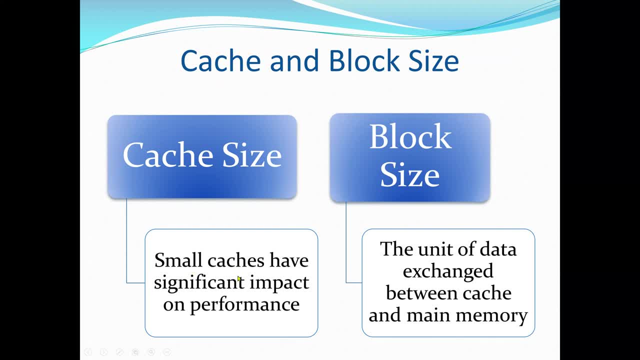 will be. the small caches have significant, significant impact on performance. as we said earlier, small caches are more closer, the cpu's more faster. then we have the block size, the unit of data exchange between the cache and also the main memory. so we have already dealt with the issue of cache size. now it turns out that there's one. 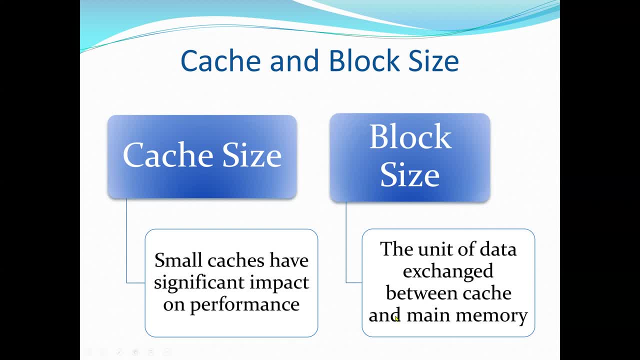 the reasonable small caches can have a significant impact on performance and also another size issue is that of the block size, the unit of data exchange between cache and main memory. so as the block size increases from very small to larger size, remember the diagram, the h, which is the. 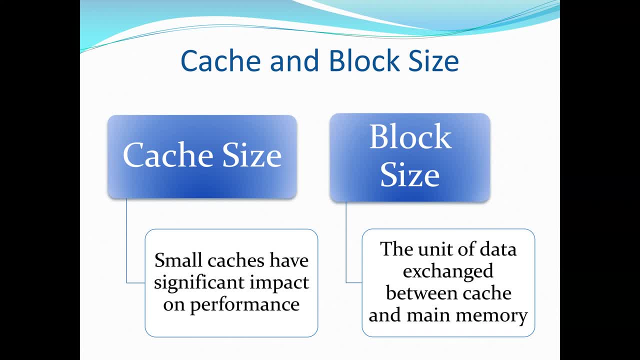 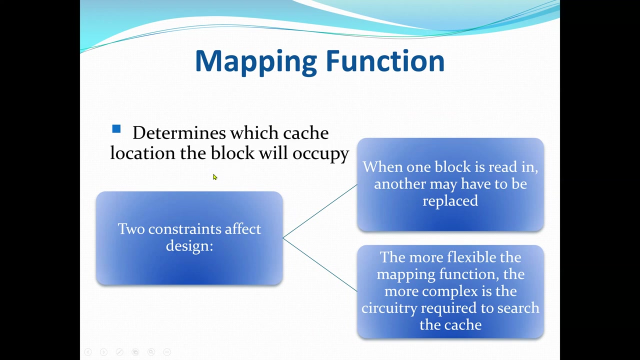 heat ratio will at first increase because of the principles of locality, the high probability that data in the vicinity of the reference world are likely to be referenced in the near future. now the next is the mapping function. here we are going to determine which cache location the block will occupy. there's two constraints affecting this design. 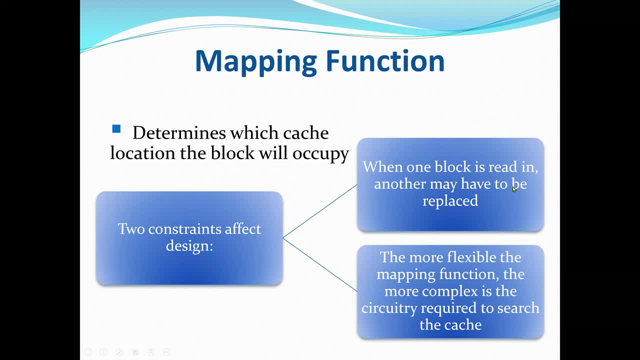 again, when one block is reading, another may have to be replaced. and also, the more flexible the mapping function, the more complex is the circuitry required to search the cache. so when a new block of data is read into the cache, the mapping function determine which cache location the block will occupy, and, as you. 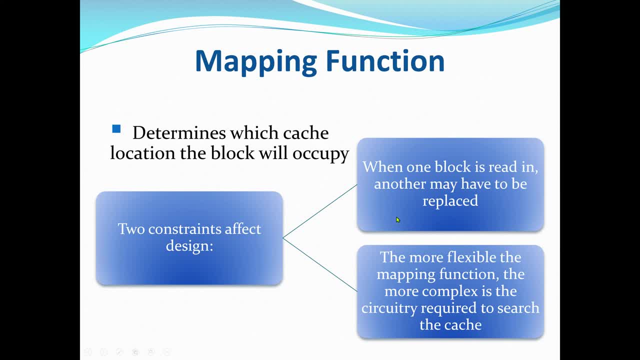 said, the two constraints here affect the design of the monthly function. first, one block is read, in, another may have to replace. we would like to do this in such a way as to minimize the probability that we will replace the block that will be needed in the in the near future. 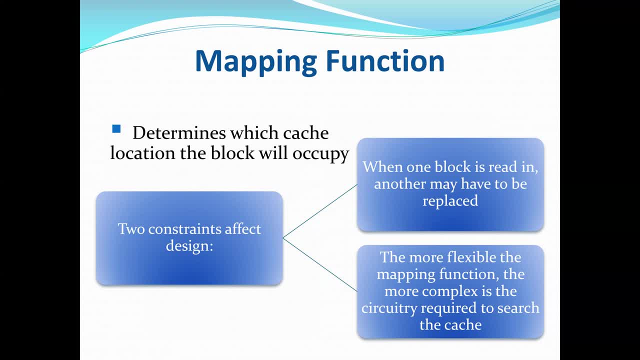 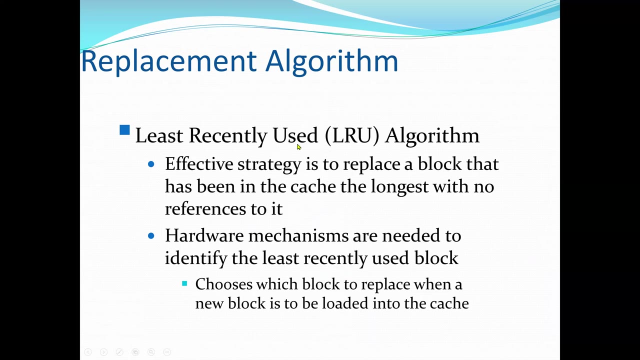 so the more flexible the mapping, match and map it function, the more scope we have to design a replacement of garraband to maximize the heat ratio And that will be the next replacement algorithm And the concept here is that the least recently used algorithm. this is an effective strategy. 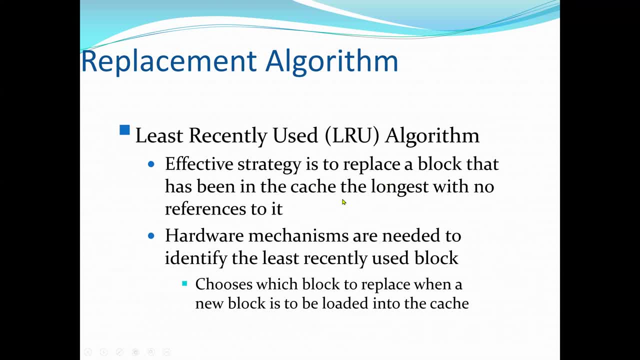 that can replace a block that has been the cache the longest with no reference to it. So the least recently used replace that And also the hardware mechanism are needed to identify the least recently used block. So the replacement algorithm again chooses within the constraint of the mapping function. 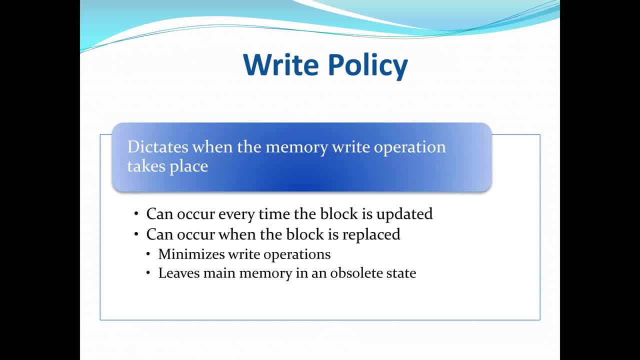 which block to replace when a new block is to be loaded into the cache. So the one that does not be used for long term, the least used one, will be replaced. Now we also have what we call the write policy. So the write policy normally would dictate when the memory 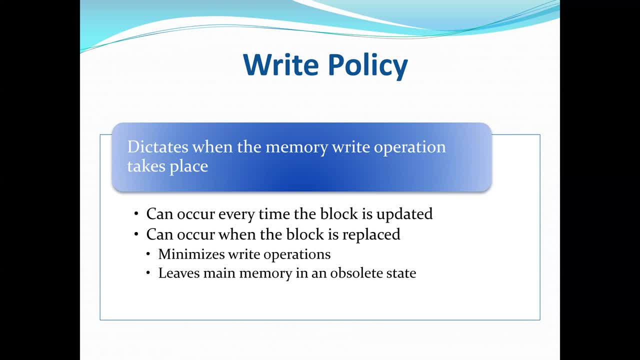 write operation takes place. At one extreme the writing can occur every time that the block is updated And at the other extreme the writing occurs only when the block is replaced. So the writing policy dictates when the memory write takes place. it can occur every time. 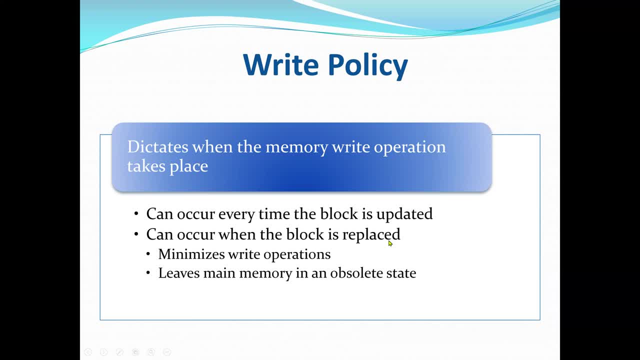 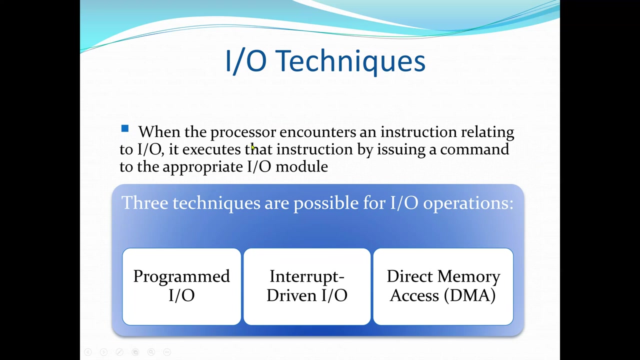 the block is updated or can occur when the block is replaced. This will minimize the write operations and also leave the memory Okay. So the next is the IO techniques, And here we say when the processor encounters an instruction relating to input and output. 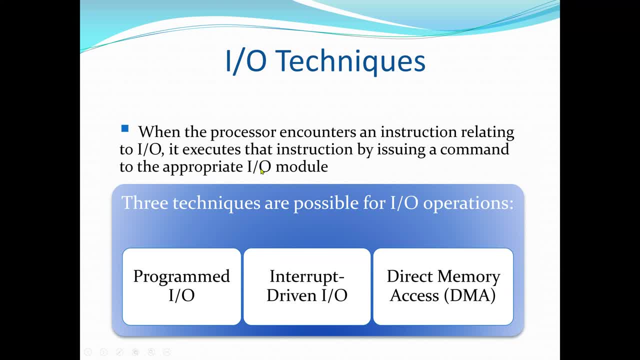 it executes that instruction by issuing a command to the appropriate input output modules. So there are three techniques that are possible for the input output operation, That is, the program input output or, if there's an interrupt, driven input output, or the direct memory address. 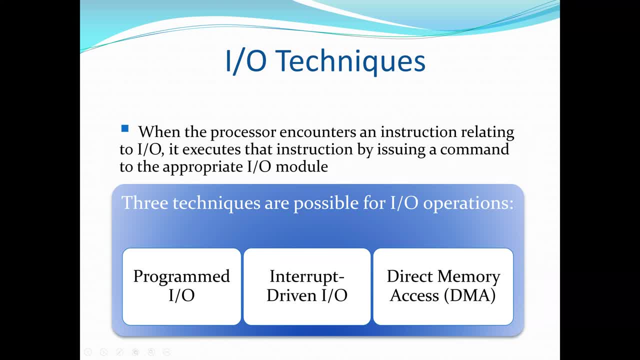 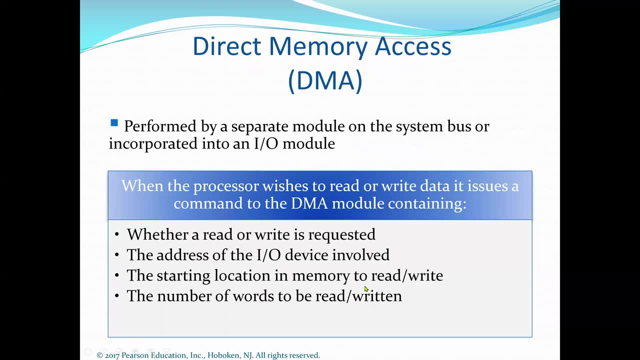 So, again, when the large volumes of data are to be moved, a more efficient technique is required, which is the direct memory address. So this is performed by separate module on the system bus or incorporated into an IO module And, as we said, when the processor wishes to read or write data, it issues command to. 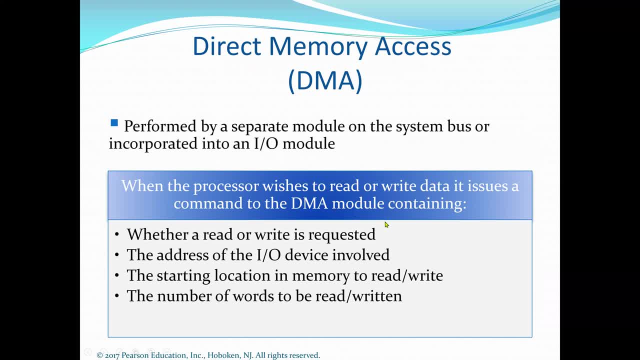 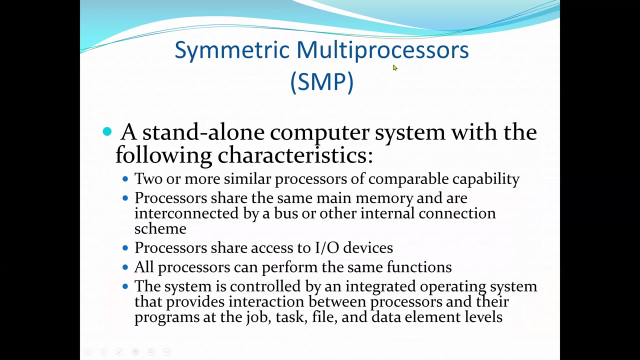 the direct memory address module, whether a read or write is requested or the address of the IO device is involved, Also the starting location in memory to read and write And also the number of words to be read and written. Okay, Okay, So this is the symmetric multiprocessors SMP. 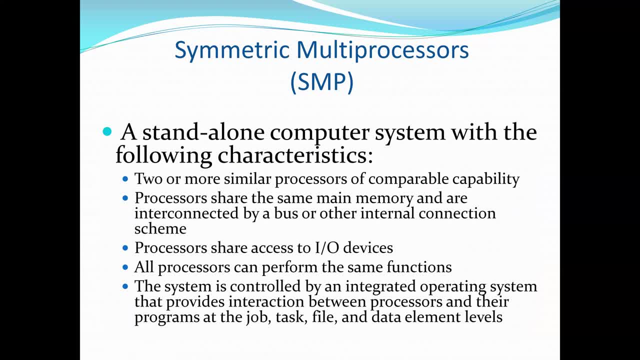 This is again the stand alone is defined as the stand alone computer system with the following characteristics: As we can see first, there are two or more similar processes of comparable capabilities. Also, these processes share the same main memory and also the input and output facilities interconnected. 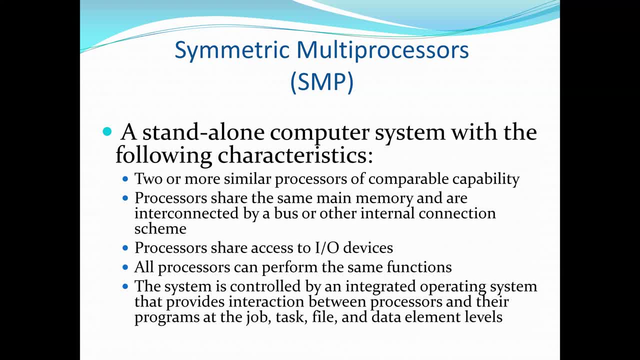 by bus or other components, For example. this is the internal connection scheme, such as the memory. access time is approximately the same for each processor. Also, all the processes share access to input and output devices, either through the same channels or two different channels that provide path to the same device. 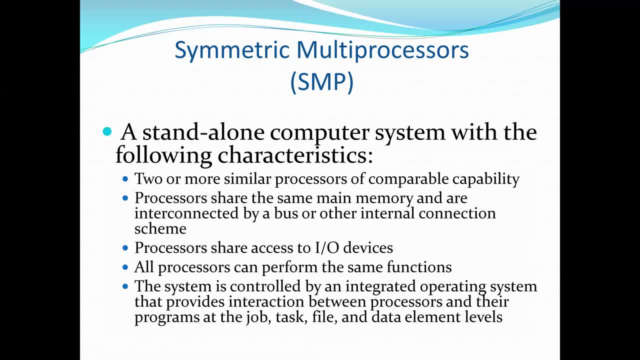 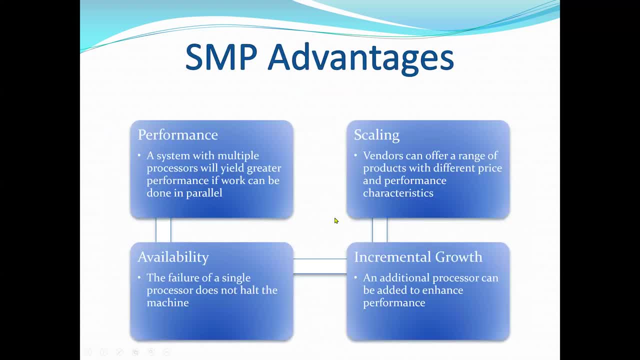 All processes can perform the same function, So that's why we say: use the term symmetric, Okay. So the first thing that we can see is the performance. Now, what are the advantages here? Performance: the system with multiple processes, of course, will yield greater performance. 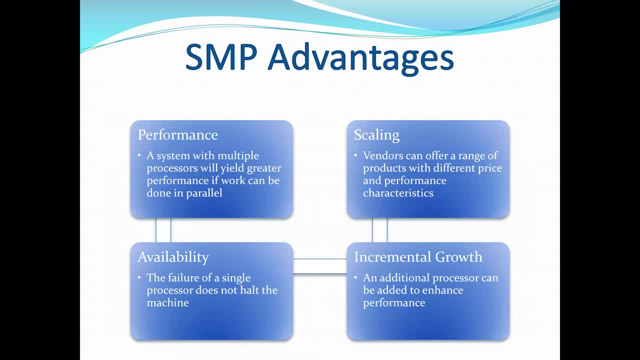 It's like you have two people building one house, 10 people building the same size of house. They will be more faster, Even though they'll be ahead of communication, but still faster. Also, scaling vendors can offer a range of products with different prices and performance. 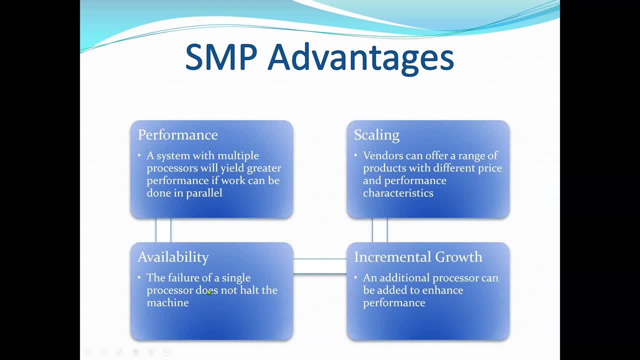 And performance characteristics And also availability. The failure of one processor does not halt the system. The other processors can again continue the work And also the incremental growth. We can have as many processes as we want. We start with two, next time can make it three, et cetera. increment it. 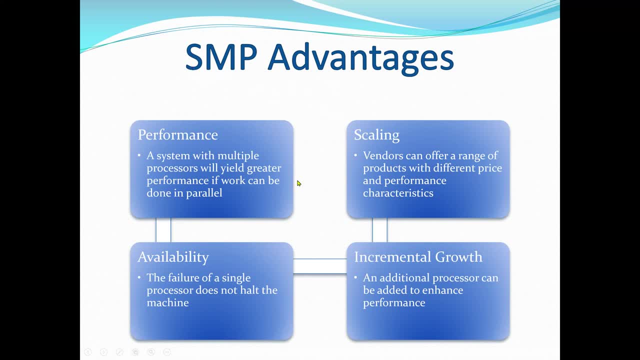 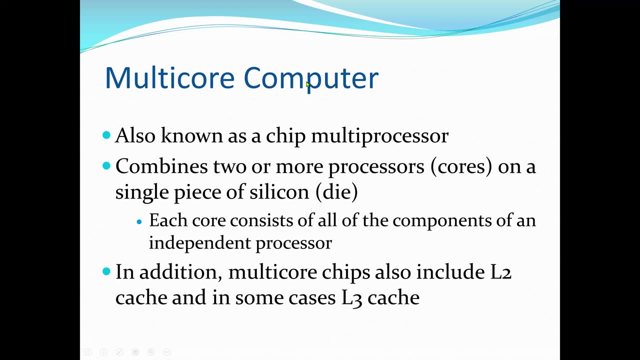 So there's a very good advantage of SMP systems. Okay, We also have what we call the multi-core computer, a multi-core computer also known as the chip multi-processor. Normally here we combine two or more processes, which we call the cores, on a single piece. 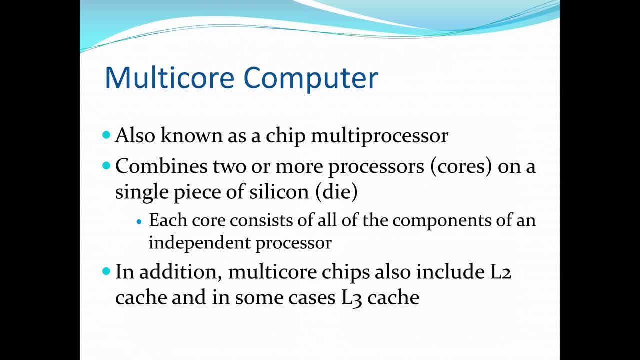 of silicon, called a die. Typically, each core consists of all of the components of an independent processor, such as the chip component, which is the chip component. Each core will have its own register, its own ALU, which is the arithmetic logic unit. 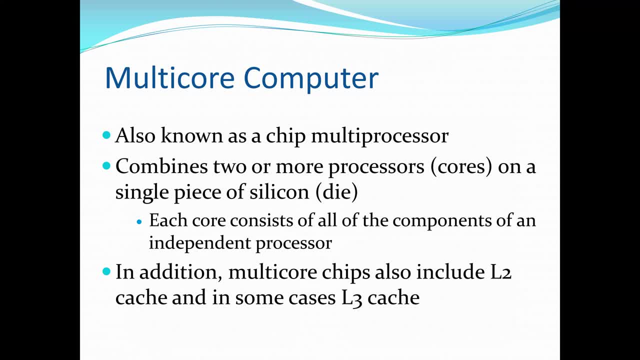 the pipeline hardware, the control units, So each processor have all the possible components, elements to perform on its own, including the caches. So, in addition, the multi-cores- contemporary multi-core chips- also include L2 cache, That's level two cache. 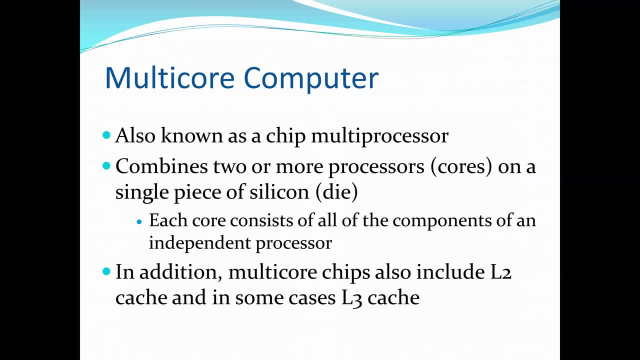 And then, in addition, the multi-cores, The multi-cores. We have all the components, the components, the components. So each processor has all the components to perform on its own level two cache. In some cases it has level three cache also. 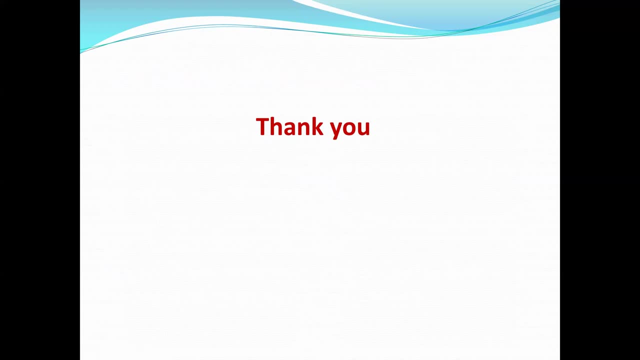 So again, thank you for these lectures. In these lectures, again, we cover the concept of memory hierarchy and also memory relationships. So, as we mentioned, the cost, the capacity, the performance, those are the three main things we need to consider. We have memory that have large capacity, but 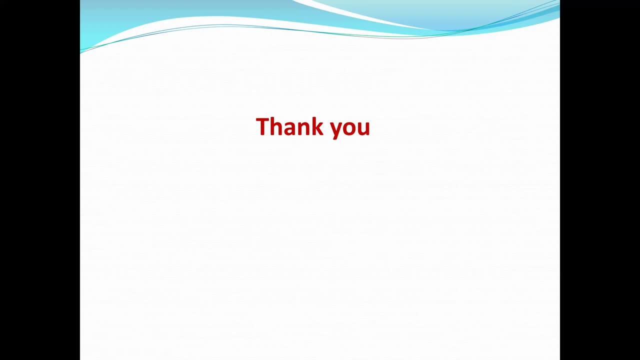 very slow and is cheaper. Memory that have high performance is very expensive, so the capacity is small. So those are the relationships between the memories. These three characteristics will define the relationship. So, for example, memory cache and register- Register is the most faster. and the most expensive. So capacity is always less, as we saw in the pyramid. Then next will be the cache, then the main memory, Then from main memory we have our secondary storage devices, the permanent hard drive, flash drive, etc. So